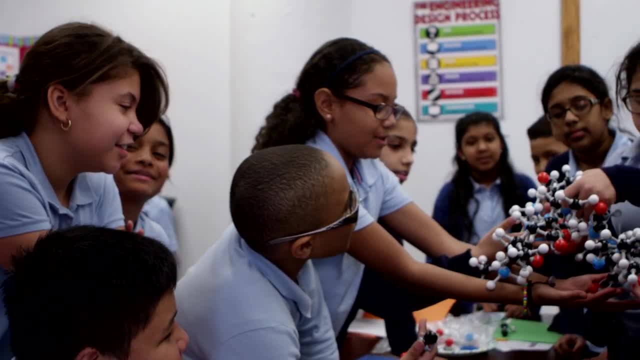 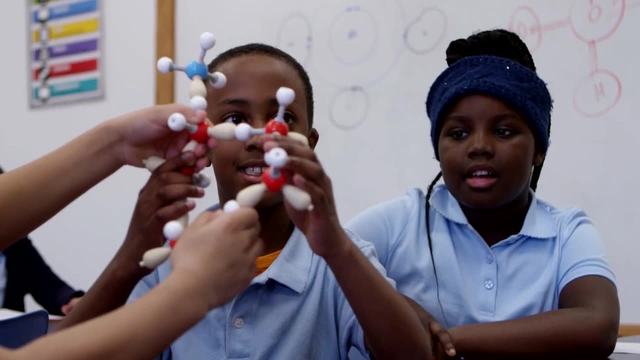 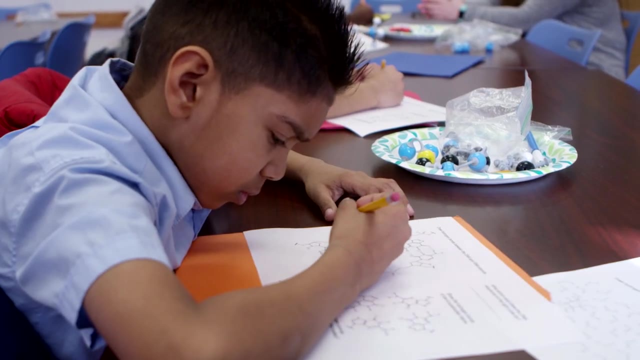 What else could be more important? And what you are seeing is how learning should be. My purpose is to prove something that I've always believed: that kids can do anything. I teach college science to kids because it's a way to show the world what's really possible. 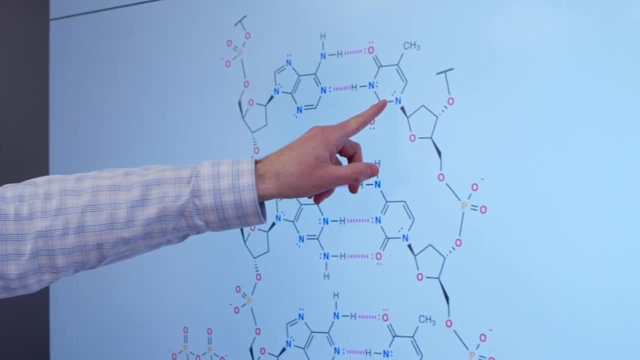 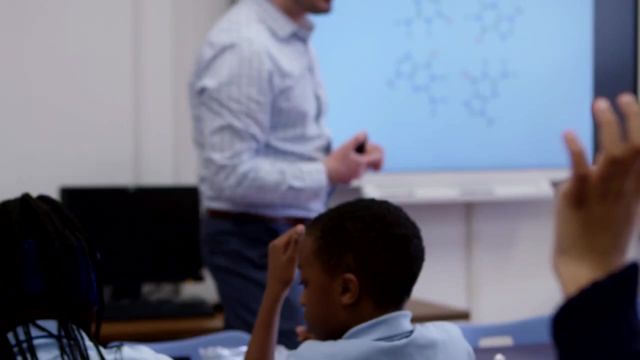 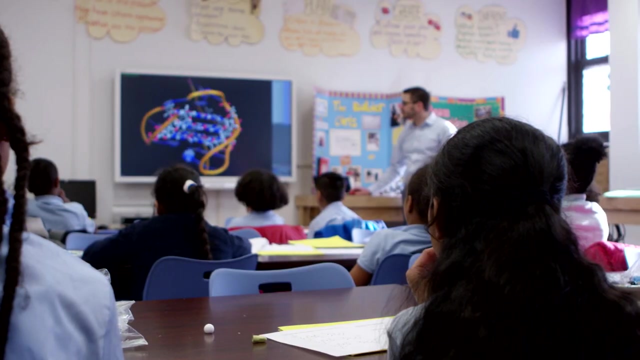 Within this room, there just might be a genius who, with a great discovery, will save us all one day. Biochemistry is the study of life at high resolution. at its most fundamental level, It answers the most basic and the most complex questions about life. 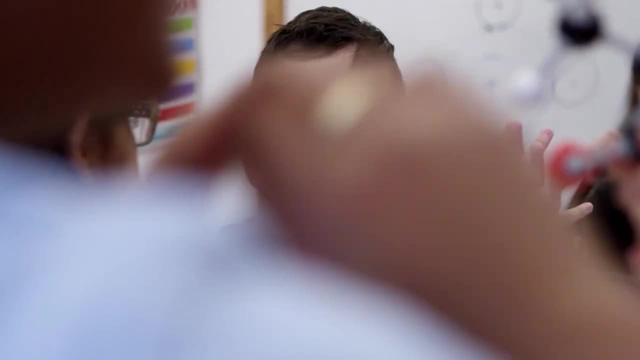 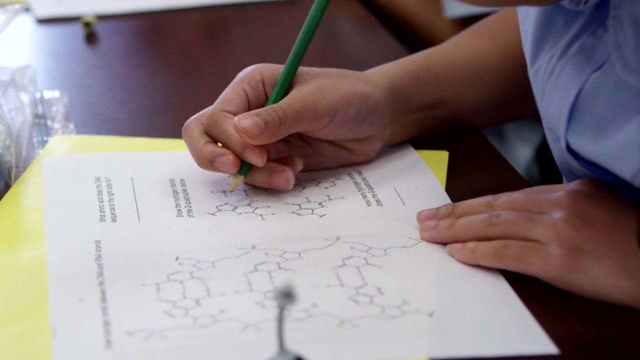 What are we made of? Why do we breathe? How do we see? How do we design our minds? We are made of medicine to save a sick person's life. For the first time in history, the answers to these questions are known, but only by a few. 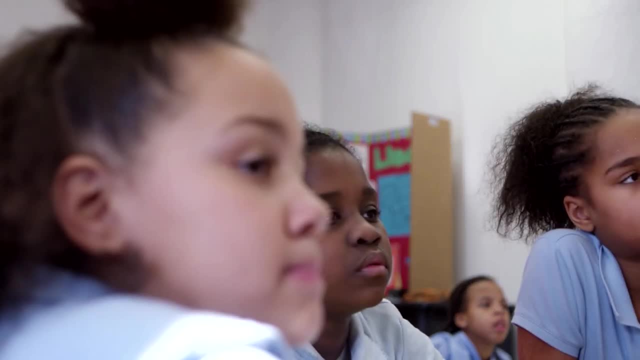 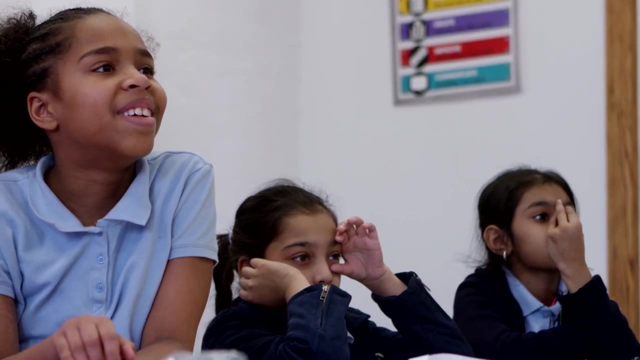 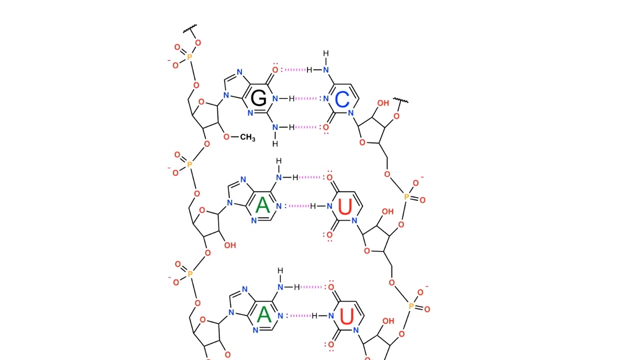 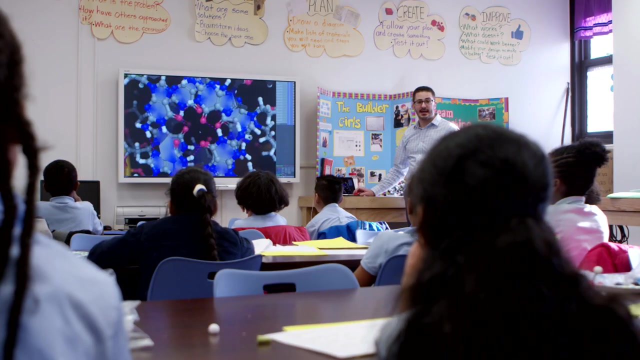 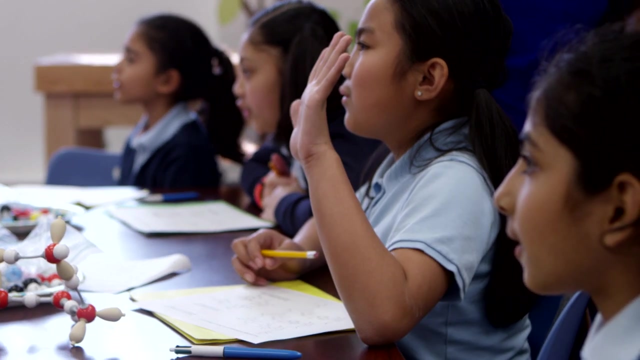 We can change that. My students learn chemistry in a way that is completely unique, as something that can be seen and touched. We interpret elaborate visualizations and build intricate models to grasp the molecular reality that underlies our living world. To design a class where kids could learn to such incredible depth and at such speed, I needed absolute creative freedom, technical knowledge and vast amounts of time. 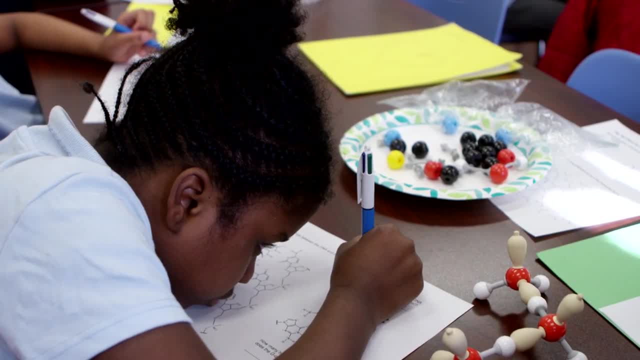 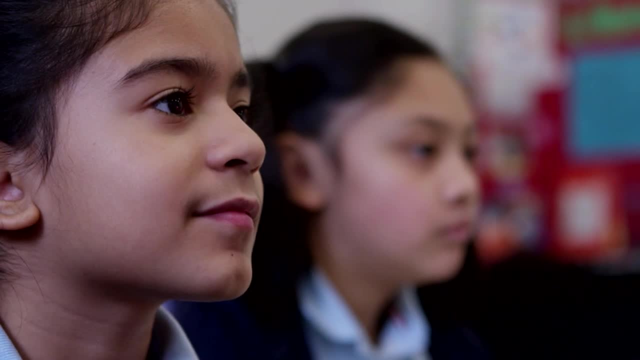 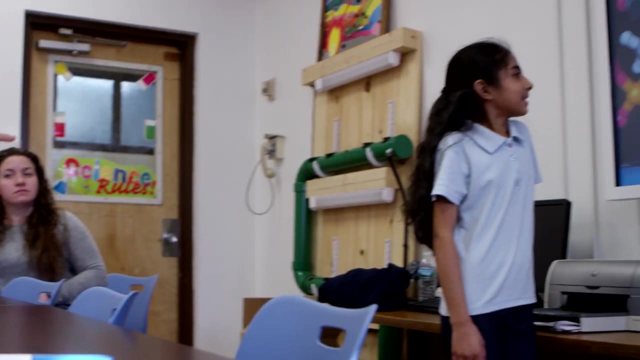 It's probably something that no one has ever been able to do before, But the most important thing that allows my students to succeed is my belief that they can, And the most important thing I can say is that I can. Here and in my mind all the time I see. I see that the world is a place in which human beings can work. 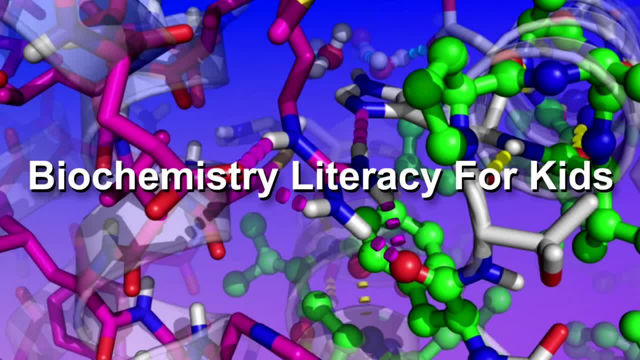 I can see that our world is part of representation, of providence, of justice, of solidarity, of love, of connection. There is a connection between the world and the world of things. It is a language that is the essence of human life. 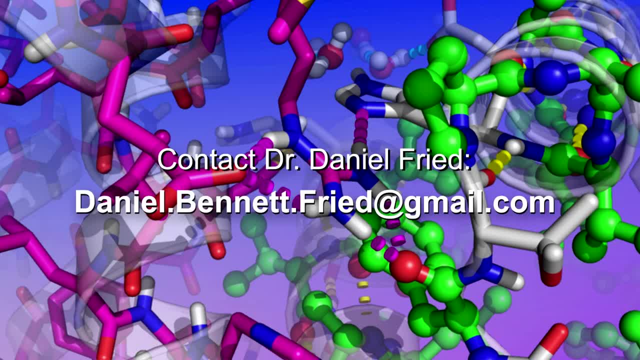 It is a language that explains how humans, humans and humans can be connected to one another. The world is a place where we have the ability to connect with one another. The world is a place where we are all connected — and all of us are dedicated to each other. 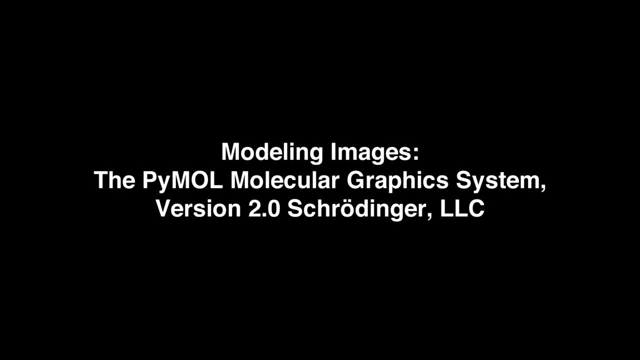 For more information, visit the FAA website. Thank you.